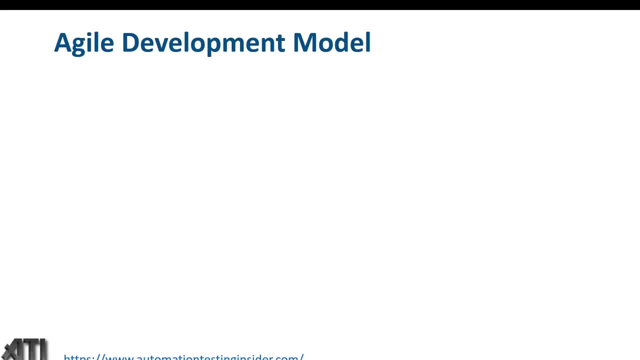 So, guys, let's talk more about Agile development model, or you can call it as Agile methodology or Agile process model. Now there are a couple of things which is very, very much important in Agile, like continuous delivery- continuous delivery of the software to the customer. 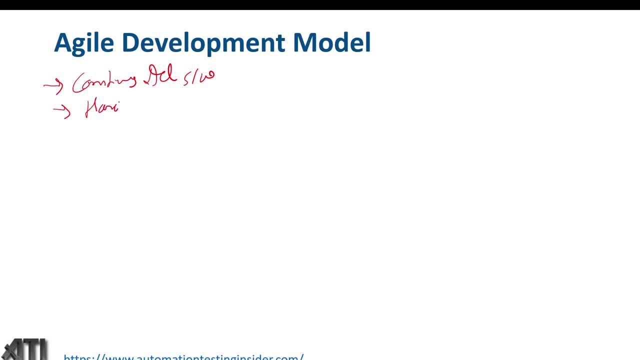 And the second thing is handle the requirement change, requirement change. So these are the two important concept of Agile development model. So, unlike in previous models we have seen, we mainly focus. I mean, we have done so much on documentation part and they are not capable enough to handle the requirement change. 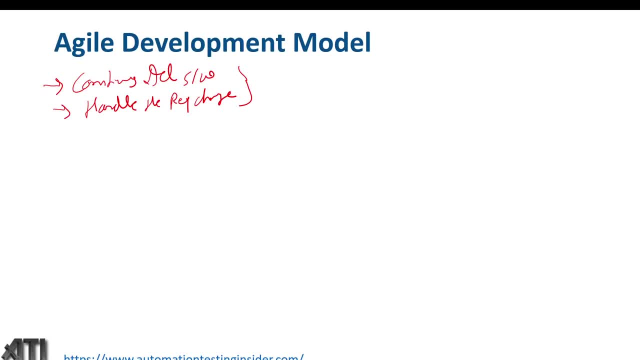 But here in Agile development model we mainly focus on continuous delivery of the software to the customer and handle the requirement change, handle the frequent requirement change in the software. So these are two important points about the Agile development model. Now there is a certain process to follow the Agile development model. 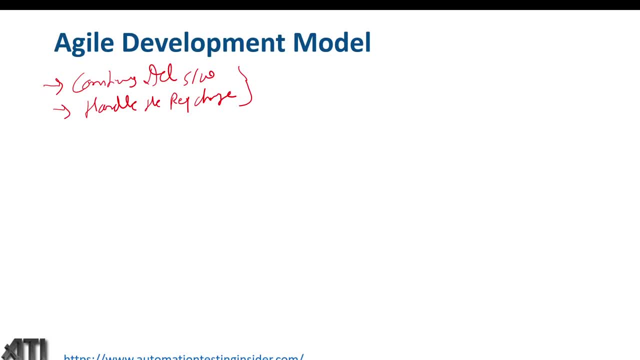 There are certain stages Now. take an example: We got the project from one customer and duration of that project is one year. Now we divide. customer wants the software in every two weeks. So we'll divide the software. We'll divide the complete requirements into different modules. 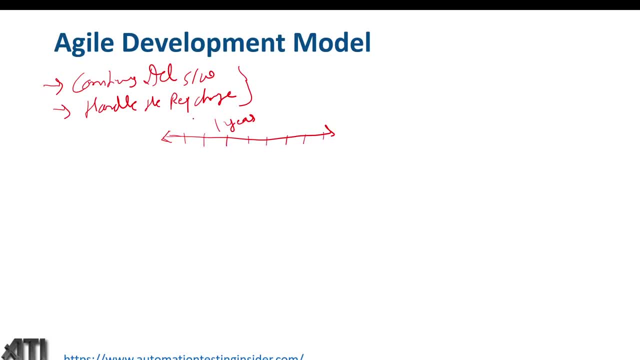 So like this. So take an example: This is X, This is Y requirement, This is Z. So we have divided the software, So we have divided the different requirements into different modules. So each module, they wants the software in every two weeks. 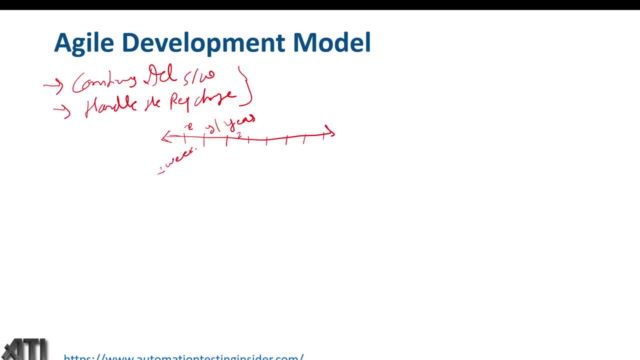 So that two weeks duration is nothing but our sprint cycle. So sprint cycle is of two weeks. So every two weeks we'll release the software to the customer. Now, in that two weeks we have to follow the complete Agile process. So what are the different steps we have in Agile process model? 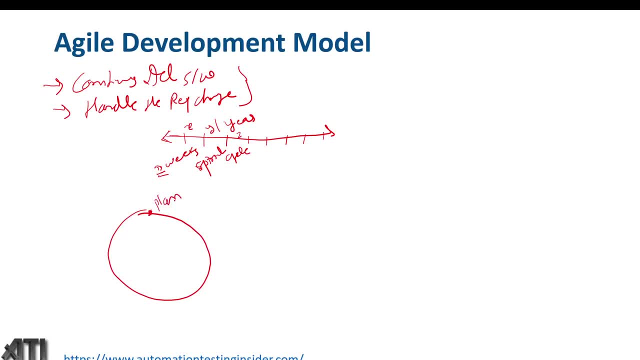 In Agile development. we have plan, planning of the sprint. We have design- Design. we have seen like high level design, low level design we have discussed earlier. And then we have development, develop and we have test Testing the software and release and last feedback. 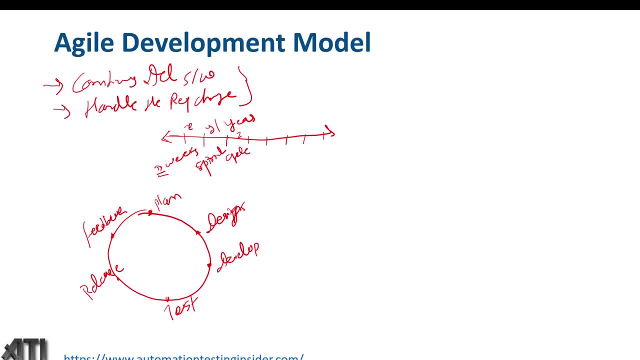 So this is the complete process of Agile development model, guys. So we have plan, planning of the particular sprint And then design. We'll do the design and development of, or coding, Development or coding- you can say Coding and testing of the software. 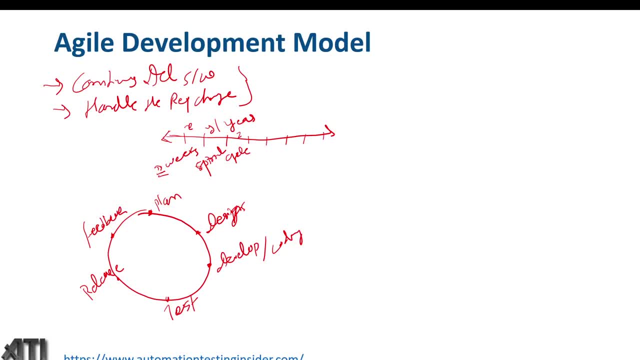 Release the software and get the feedback from the customer Now. so this Agile development model is also called iterative. I mean it is the combination of iterative development plus incremental Incremental. Why it is iterative? Because what do you mean by iterative? 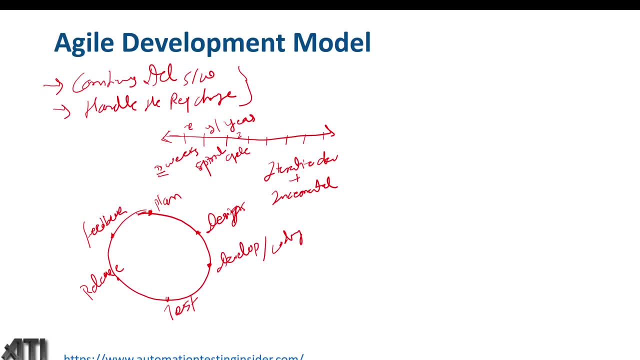 So we have seen in iterative development model, When we keep doing the same thing again and again is called iterative. So this is my model one or sprint one. So we have followed plan design, develop, test, release and feedback. Similarly we'll do for this sprint one. 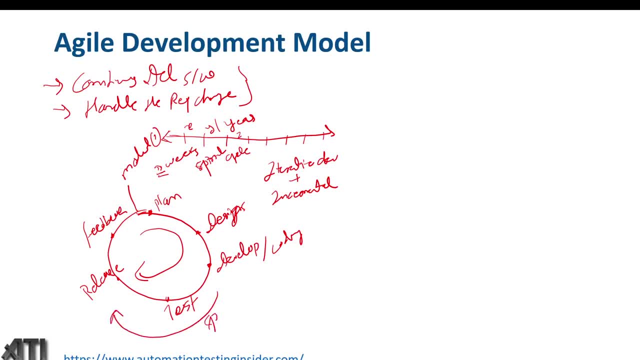 Now we'll follow the same for sprint two as well. Sprint two cycle or module two. So that's why it is iterative development model plus incremental, Why it is incremental. So we have divided our task into different modules. We have divided our task into different modules. 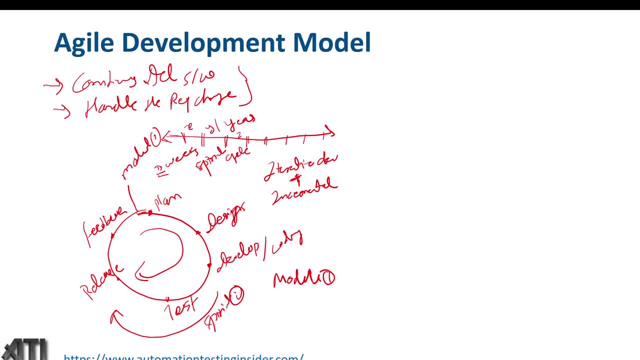 So this is module one. We made some changes on module one. I mean, we have developed some module, We have developed some requirements on module one And we'll add in module two. So we'll keep adding our requirements till we get the final project. 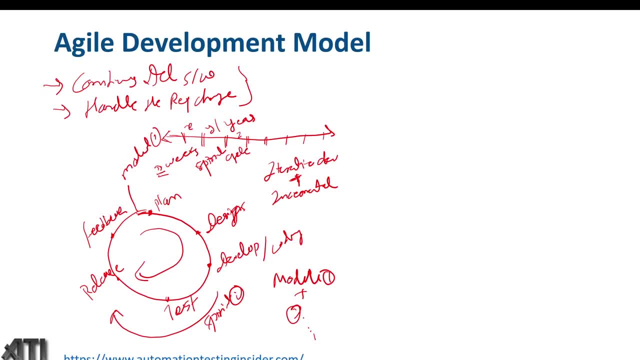 Final product. So this is kind of incremental: Module one plus module two, module three, Like that. So that's why it is incremental model as well, So it is iterative plus incremental. Now there are few terms, guys. Few terms and different meetings are there in agile development model. 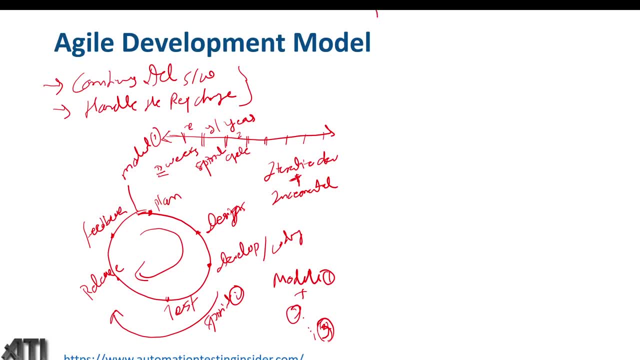 So let's talk about them in detail. What are those different? What are those different terms? we have So sprint, we have discussed Sprint, So it is nothing but the modules. We have divided the task into different modules And each module is of two weeks. 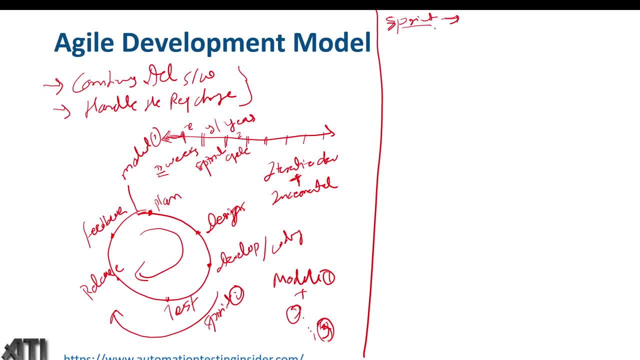 So that is nothing but the sprint. We'll plan, design, develop, test, release and get the feedback. So this is sprint. Now we have scrum. What do you mean by scrum? Basically, in agile process we have? I mean to follow the agile process. we need to follow certain framework. 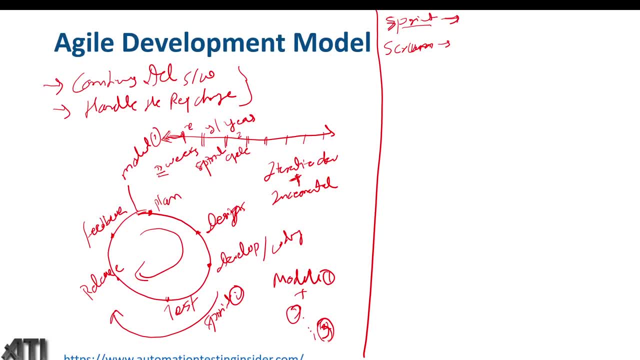 So scrum is nothing but a framework that helps the team work together, Or it is a work culture to follow the agile development model. So that is scrum. Now in scrum we have scrum master Before that: product owner. Product owner. 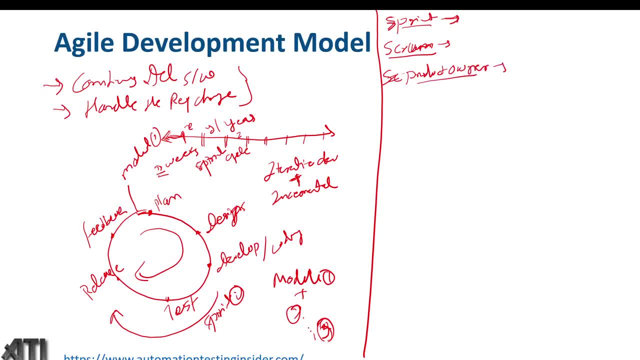 So who is the product owner? So it could be the head from the marketing team Who deals with the customer, Or it could be from top management individual as well. So who handles the requirements from the customer, Who talks about the product with the customer, is called the product owner. 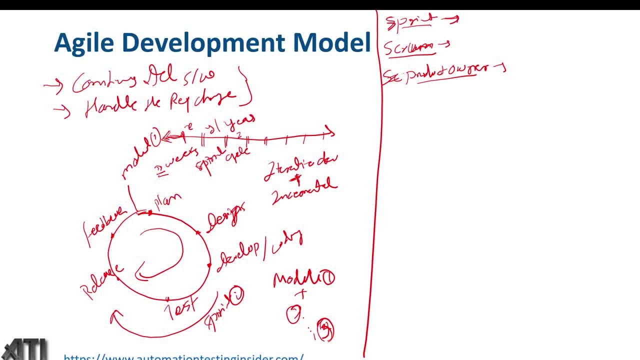 Now we have scrum master, Scrum master. So what do you mean by scrum master? So it can be project manager or project manager can be scrum master. But the difference is project manager handles different projects at the same time And scrum master is particularly for this particular project. 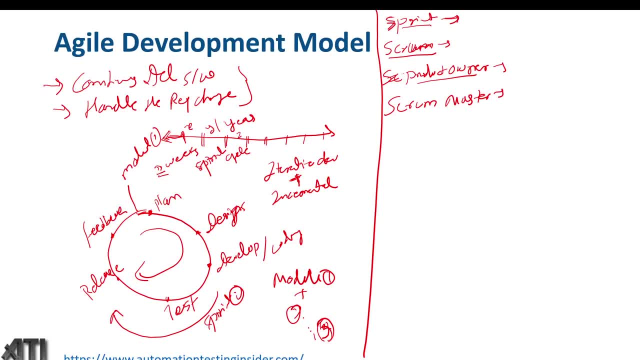 For this particular scrum. So that is scrum master. Now we have user stories. What do you mean by user stories? User story? So user story is nothing but the requirement which we got from the customer. Like, we have divided them into different sub requirements. 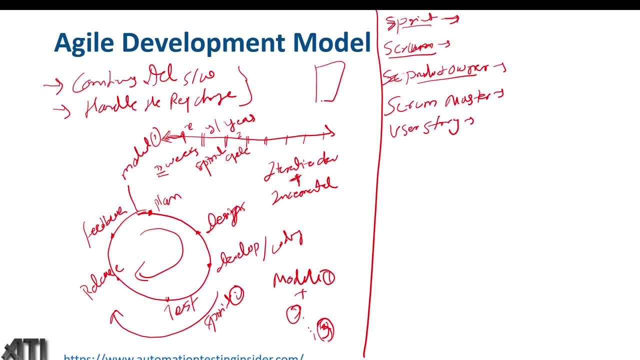 We got requirements from the customer And we have divided them into different features: X feature, Y feature, Z feature. So one user- I mean one user story- could be combination of two features or one feature, Or it could be one plus two feature. 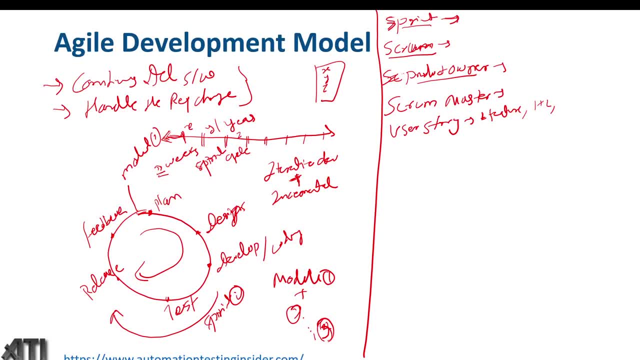 If it is like small feature, then it may have only one feature. If it is like- Sorry, If it is big feature, then it may have only one feature. And if it is kind of small requirements, If you have small requirements, Multiple requirements. 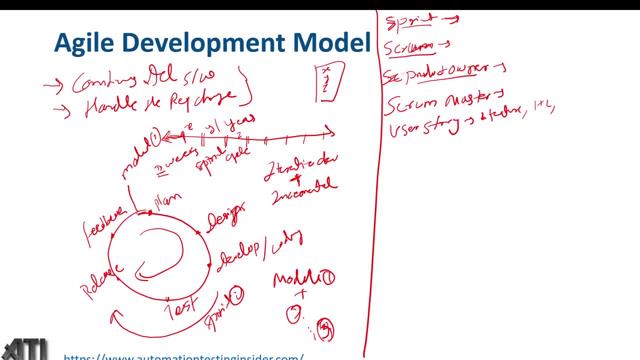 Then it could be multiple features. So that is nothing but the user story. Now what next? we have product backlog, Product backlog. So what do you mean by product backlog? So product backlog is nothing but the combination of different user stories We keep in the product backlog. 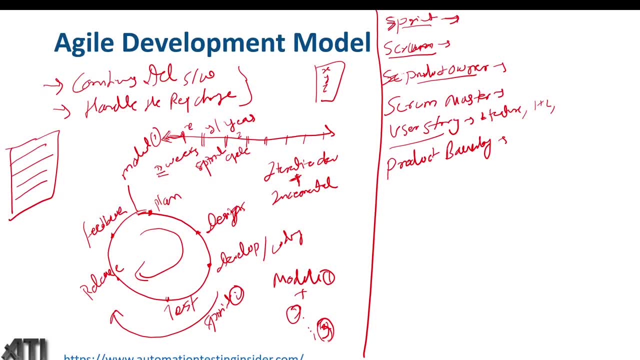 From there we will pick and plan for the particular sprint To develop that requirement. So that is product backlog. You can say: the requirements are split into user stories For any particular sprint And user stories are picked from the product backlog. Now what is next? 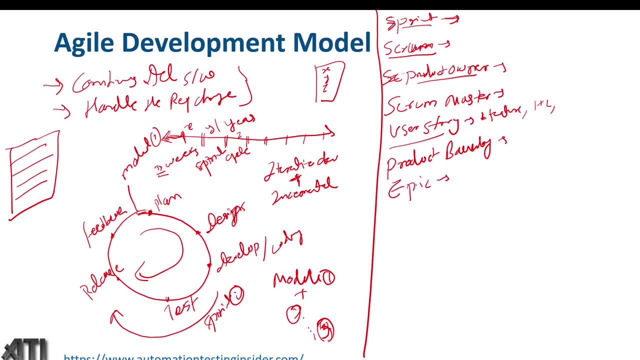 We have APIC, APIC. What do you mean by APIC? So APIC is kind of again the same thing, But it has large number of requirements In APIC. We have large number of requirements in APIC And this product backlog is for particular sprint. 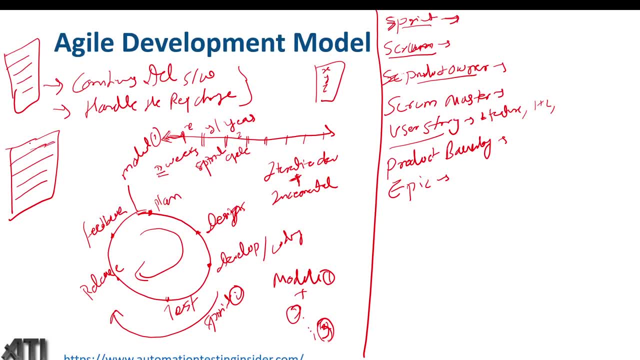 We keep all the user stories there And we pick it from here. But whereas the APIC contains different, Different requirements, We contain- It is also combination of different user stories, But maybe For different sprints, Like sprint 1, 2.. 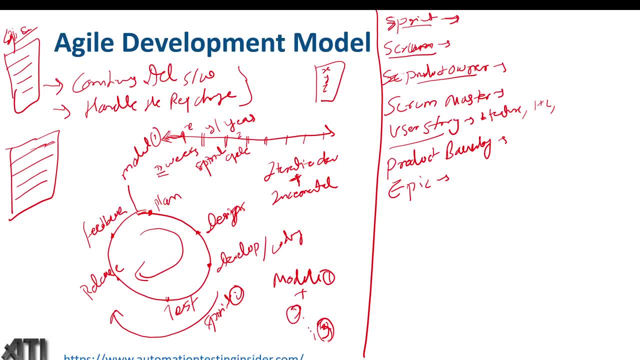 It contains all those requirements in APIC. Another point is story, Story point. Another term is story point. So what do you mean by story point? So it defines the complexity of the user story. It defines the complexity, Complexity of the user story. 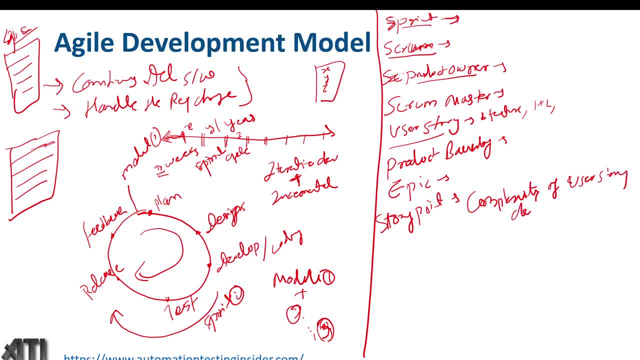 User story With respect to Team And testing team, Like how complex the particular user story. And. And The next thing is swag. Another term is called swag, So basically, in swag, What happens is It is. 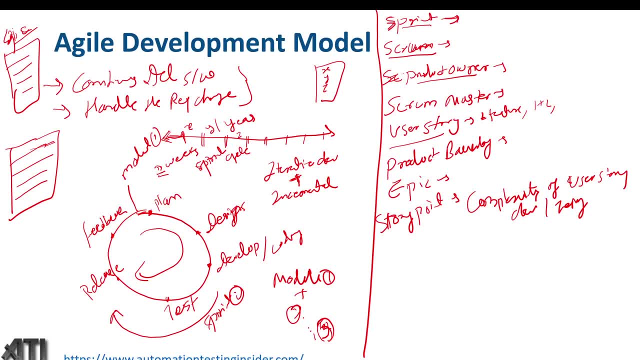 It is the way to, It is way to compare the Size, Time And effort: Size, Time And effort. So basically, in swag, What happens is It is. It is the way to, It is way to compare the. 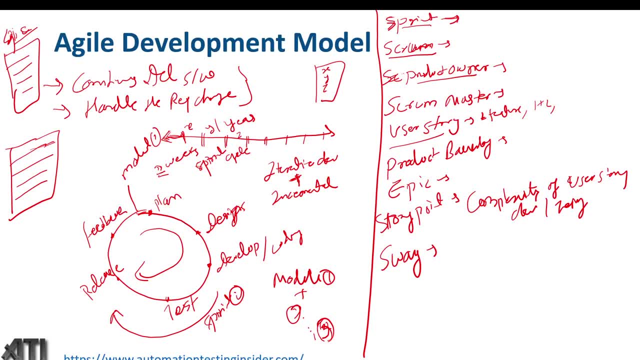 Size, Time And effort. Size, Time And effort To develop any particular User story. Size, Time And Effort. Now We conduct different Meetings, guys, So one of the meeting is Sprint Planning. 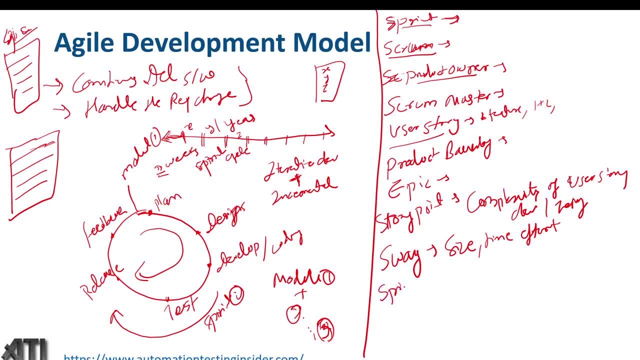 Meeting: Sprint Planning Meeting. So what do you mean by Sprint Planning Meeting? So Scrum Master Conducted This Meeting. So You Conducted This Meeting Before The Start. 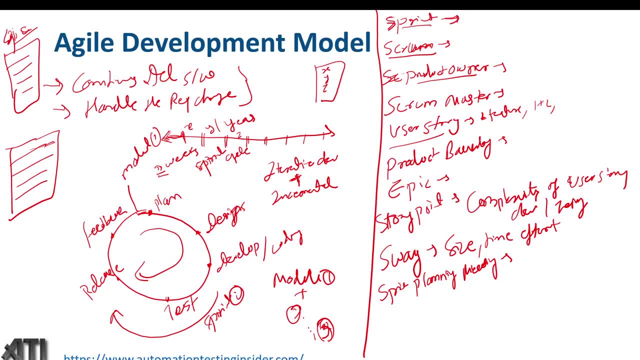 Of The Sprint To Discuss About The User Story That Can Be Covered In Particular Sprint And The Timeline Of The Same Time. So It 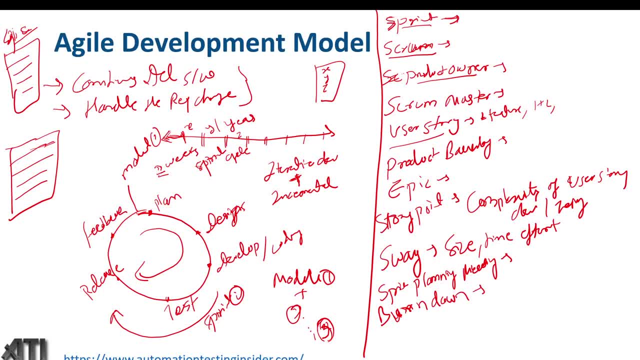 Is The Work Between Time And Work Which Shows That How Much Work Is Remaining For The Project. It Is Shows That How Much Work Is. 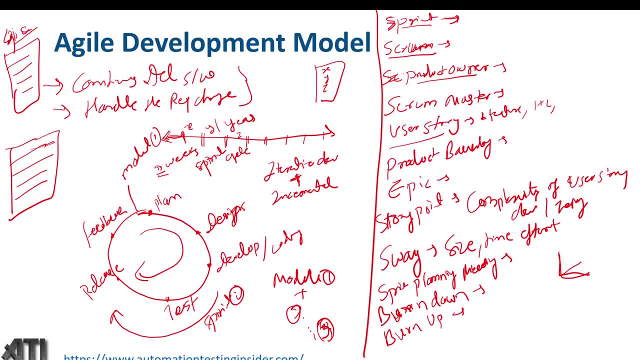 Done, How Much Work Is Done, How Much Work Has Been Completed Is Called The Burn Up And Whatever, How Much Work Is Remaining Is Called. 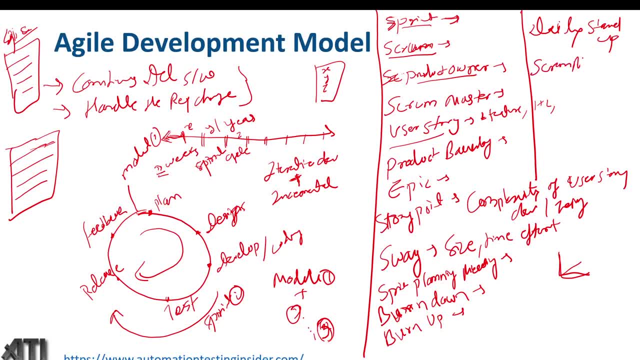 Burn Down Now Scrum Meeting. So What Happens Here Is Every Day. We Need To Have This Daily Standup Meeting Where We'll Discuss Like 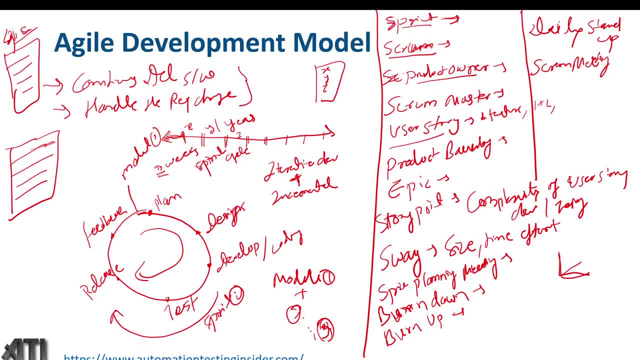 How Much Work Has Been Done Yesterday, What We Have Done This Meeting. But Scrum Master Conducting This Meeting To Discuss About The Progress, About. 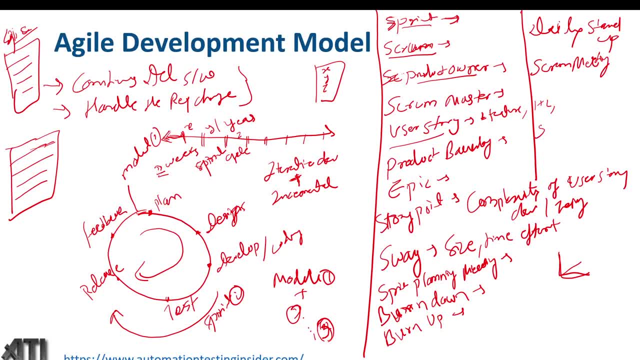 The Project And We Have What Else We Have. A Sprint Review Meeting Is Conducted At The End Of The. Once Sprint Is Completed, We 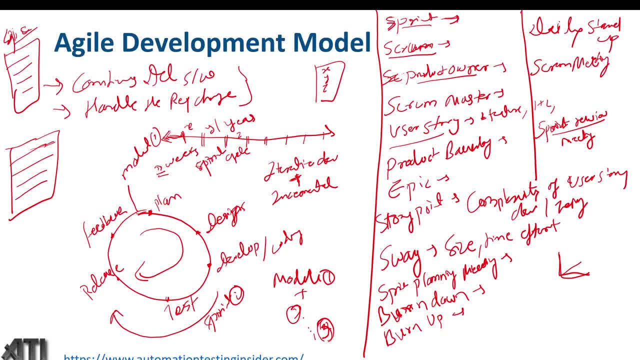 Conduct This Sprint Review Meeting, So Where We'll Discuss About How I Mean How It Was The Sprint Retrospective, Retrospective Meeting, So What? 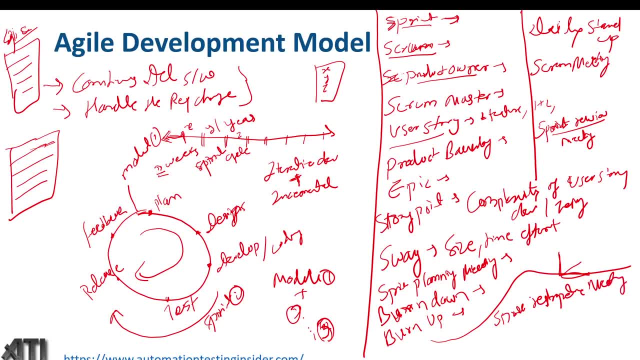 Happens In This Sprint Retrospective. So At The End Of The Sprint Or When We Have Started The New Sprint, We Conduct This All. 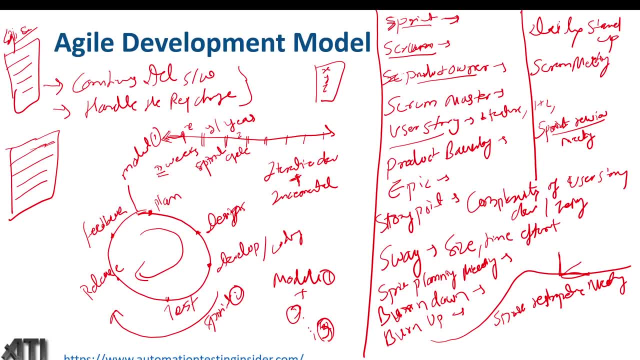 These Things Discussed In This Sprint Retrospective Meeting And At Last We Have Defect Triage Meeting, Defect Triage Meeting. So What Do? 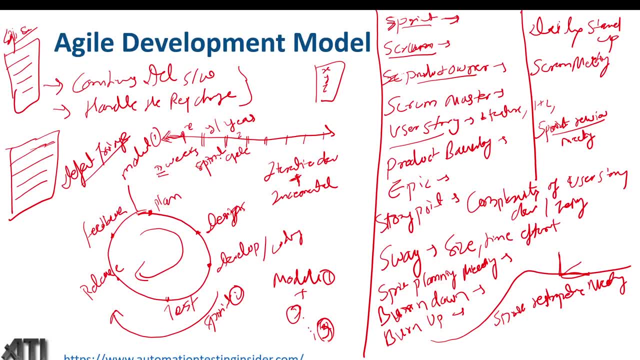 You Mean By That Defect Triage Meeting In This Particular Meeting. The Dev Team Testing Team, Product Owner Is Also Join This Meeting And 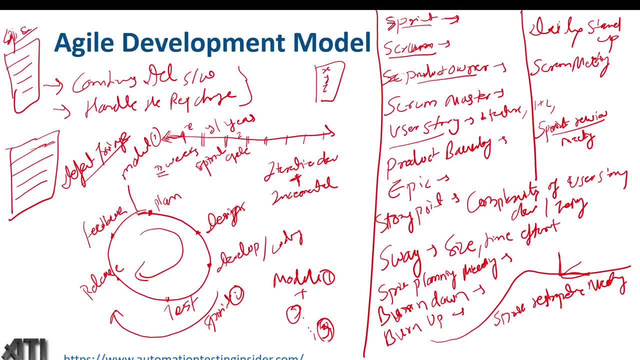 We Have A Scrum Master, So Here We'll Discuss About The Progress And Defer It To The Next Sprint. Is Not Important, But Do? 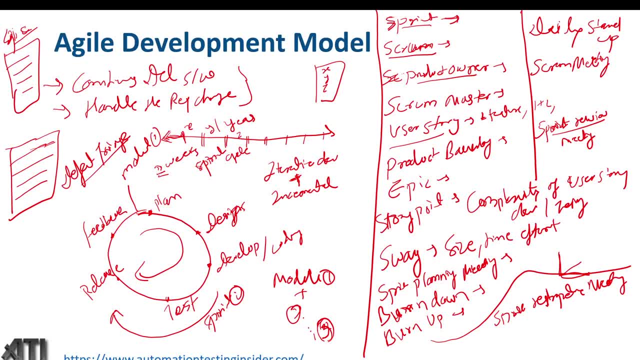 Not Worry About The Defect Related Things, Guys, Like What You May Be Defer The Defect, Or So In The Next Slide I'll 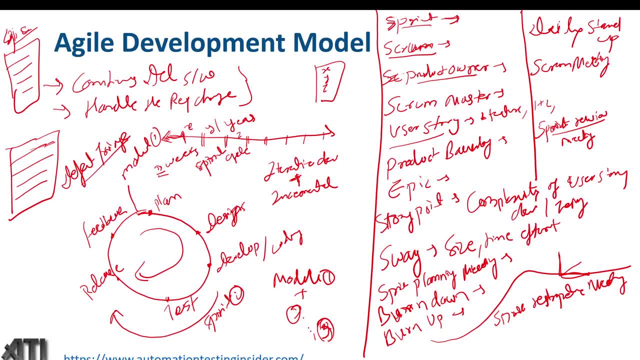 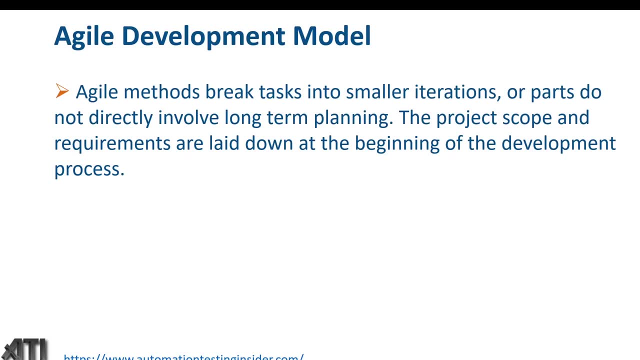 Revise, Like Whatever We Have Discussed So Far. Guys, Most Of The Points I Have Covered In This Particular Slide, But I Have Asked 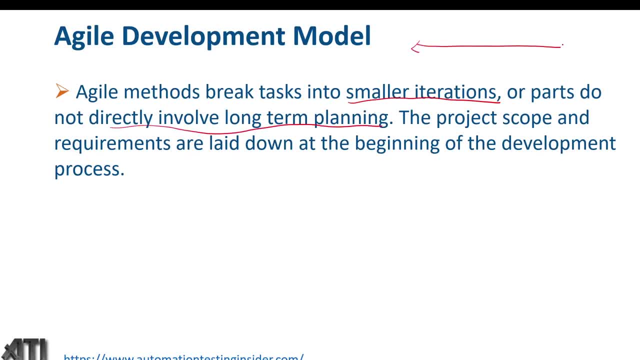 To Directly More Long Term Planning. We Have Seen One Complete One Year Project. The Project Scope And Requirements Are Laid Down At The Beginning. 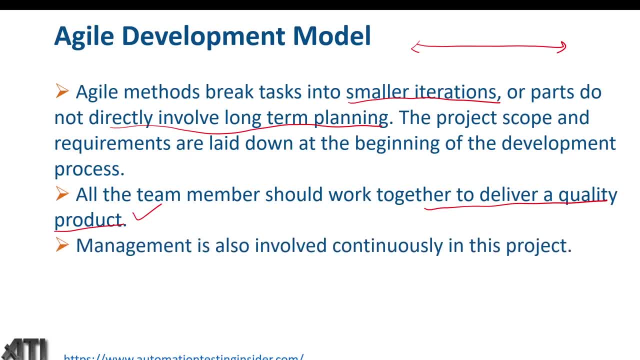 Of The Development Of The Process, Of The Development Of The Process, Of The Development Of The Process To Follow The Complete Project. It Is One. 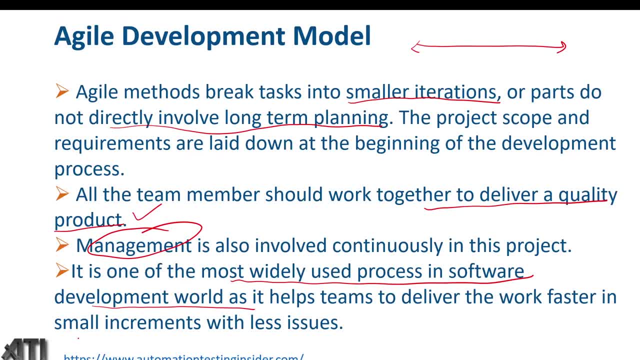 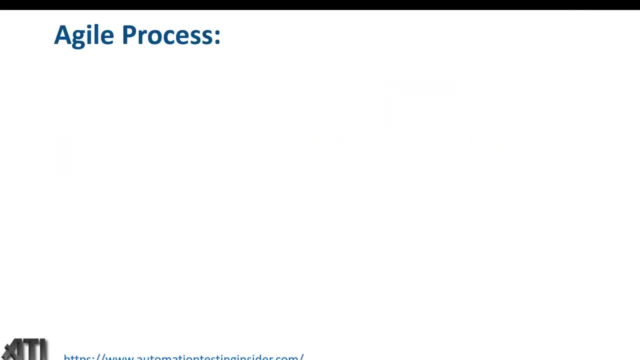 Of The Most Widely Used Process Of Agile Development Model. Now We Will Just Recap What We Have Done In Agile Process. So, Customer, Customer. 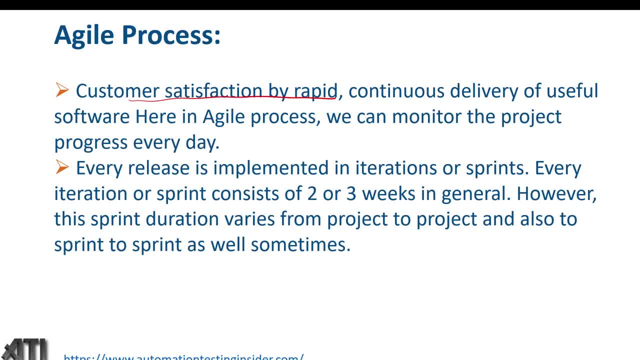 Satisfaction By Rapid, Continuous Delivery Of Useful Software Here In The Agile Process In Agile Process Is A Very Important For Agile Process In Agile Process. 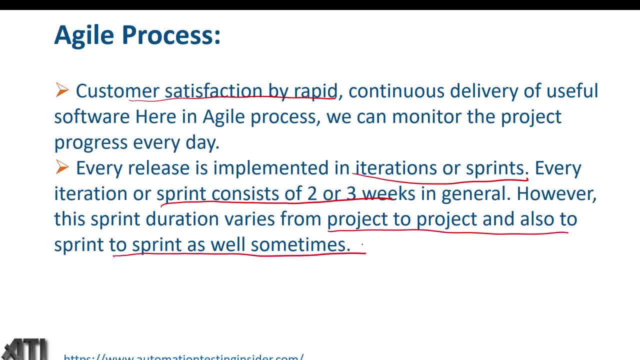 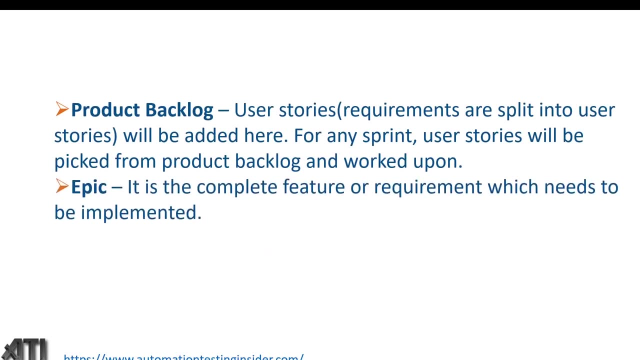 In Agile Process. Now We Have This Agile Process To Know The Process. now these are the different terms, guys, which we have already talked about. like product backlog, user stories- requirements are split into user stories will be added here in product. 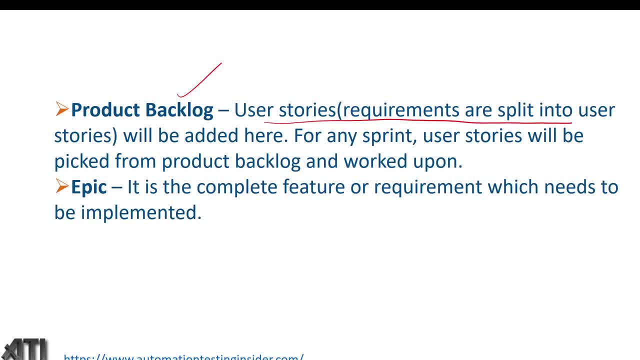 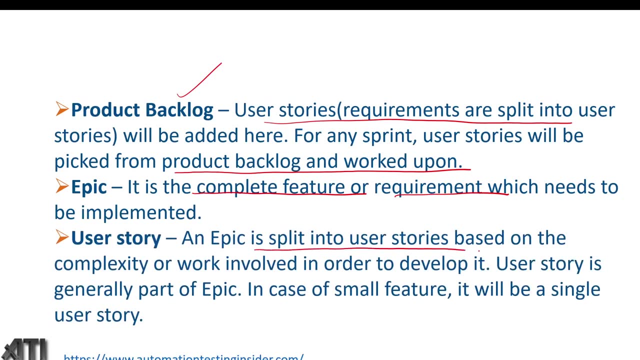 backlog for any particular screen. user stories will be picked from product backlog and worked upon epic. it is the complete feature or requirement which needs to be implemented that we have discussed. user story and epic is split into user stories based on the complexity of work involved in order to develop it. user story is generally part of epic, so we have seen. 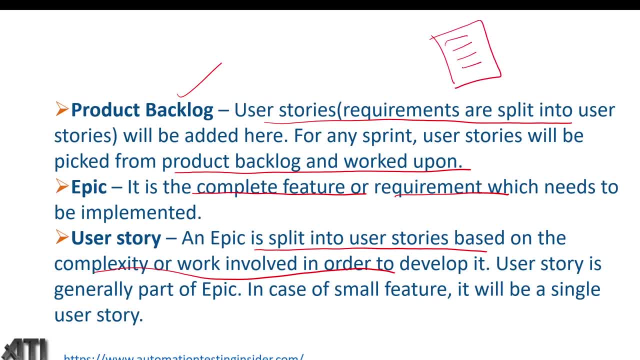 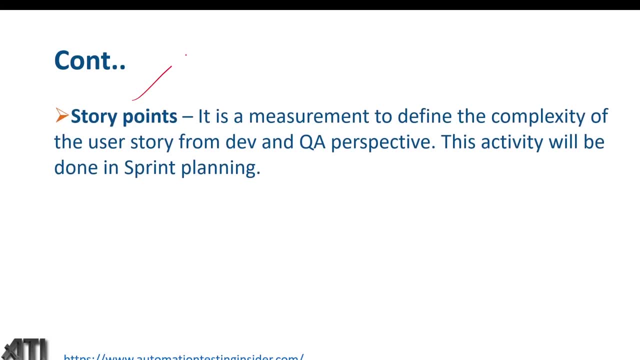 in epic we contains all the different user stories. in case of a small feature it will be a single user story. story points also we have discussed. so it is my measurement to define the complexity of the user history from dev and qa perspective. so basically, what do you mean by story points? so it defines the complexity of the user history how. 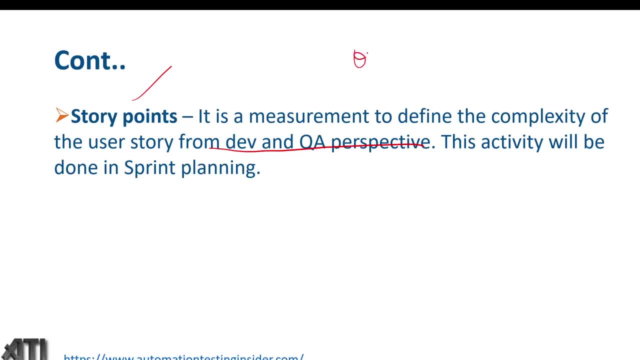 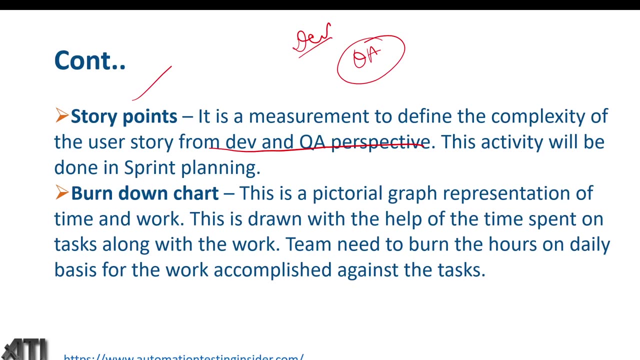 how complex is for development of that particularly particular user story and how, how complex it is for testing purpose. so this activity will be done in sprint planning. burn down chart. so we have seen burn down and burn up. so this is pictorial representation of time and work. pictorial representation of time and work. time and work team needs to burn the. 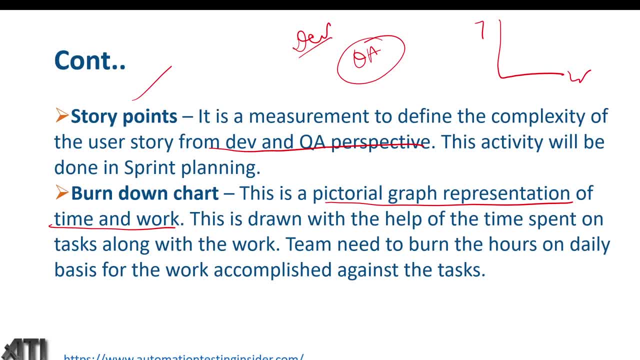 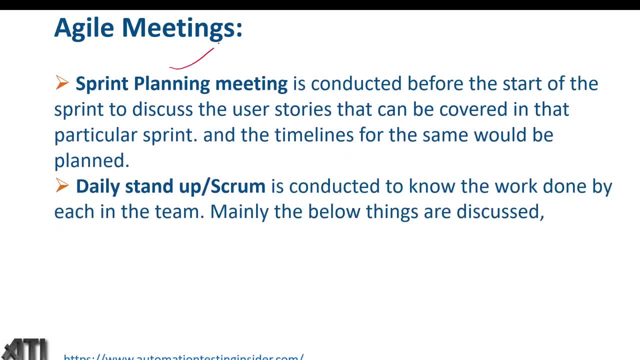 hours on daily basis for the work accomplished in the task and different agile meetings. also we have discussed so sprint planning meeting at the beginning of the sprint cycle we used to conduct the sprint planning meeting, conducted before the start of the sprint to discuss the user story and 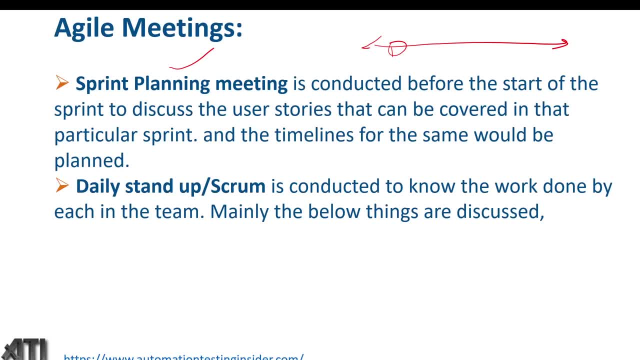 that can be covered in the particular sprint and the timelines for the same would be planned: Daily stand-up or scrum meeting. it is conducted to know the work done by each in the team. mainly the below things are discussed. so what work we have done yesterday? what work is planned for today? what work is planned? 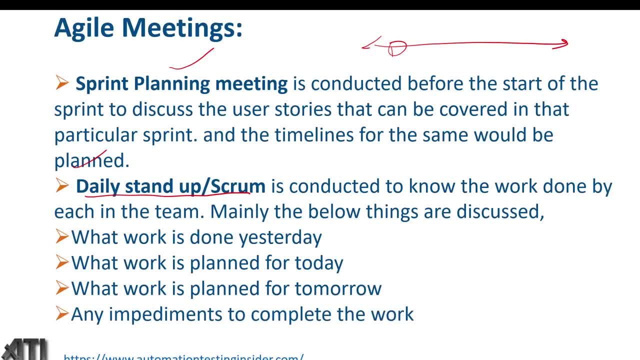 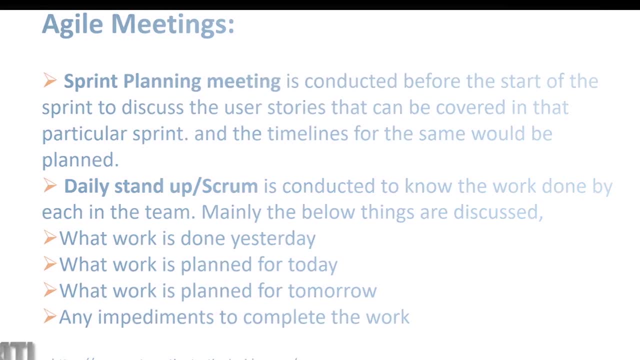 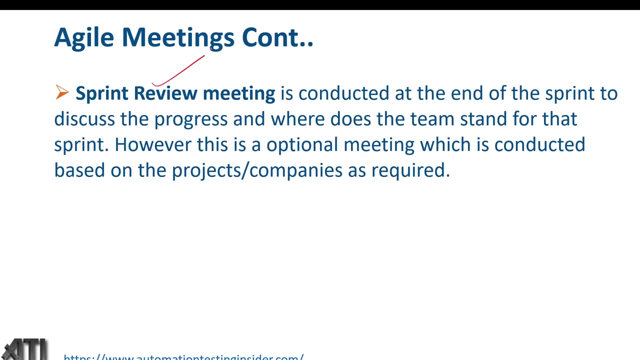 for tomorrow and any impediments to work to complete the work. impediments means any obstacles or any problems we are facing to complete the work. will discuss, will be discussed- discussed in this particular daily stand-up meeting and sprint review meeting is conducted at the end of the sprint to discuss the 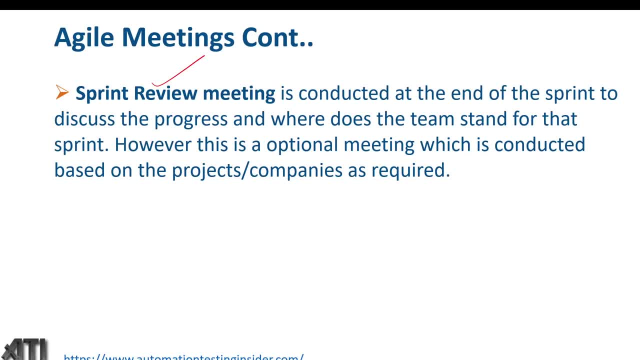 progress and where does the team stand for the sprint. However, this is optional meeting, as I have discussed earlier, which is conducted based on the project companies as required Sprint retrospective meeting. so this is an important point, or important meeting is conducted once the sprint is completed and next sprint got started following: 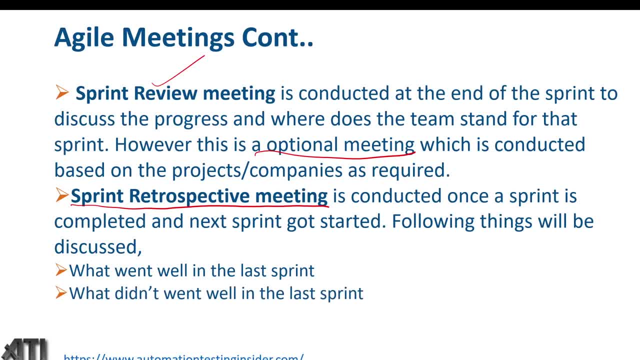 things will be discussed like what went well in the last sprint, what didn't fail the last sprint and what can be done to improve or perform well in the ongoing sprint. These are the points which we discuss in retrospective meeting, Defect triage meeting. so this is an important meeting. it's conducted to 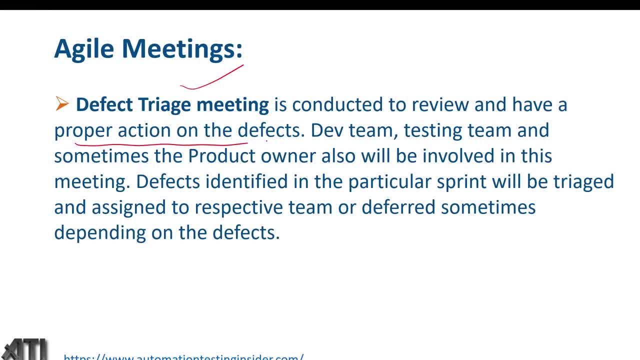 review and have a proper action on the defects which I talked about. Dev team, testing team and sometimes product owner also will be involved in this meeting. defects identified in the particular sprint will be triaged and assigned to respective team or deferred sometimes, depending on the defects. So sometimes 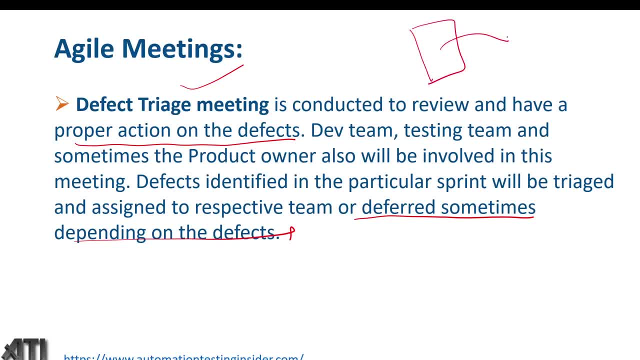 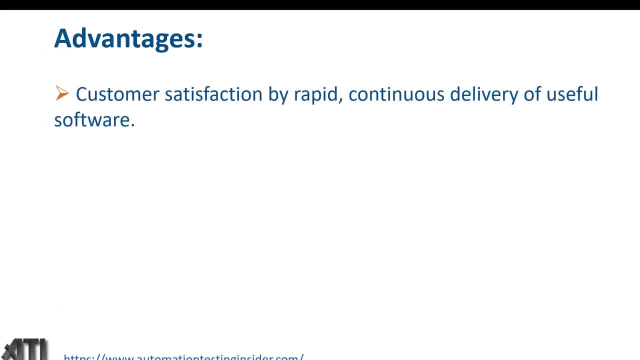 any defect is not important to fix, So we'll defer it for the testing if need to. Next is Sprint. What are the different advantages of Agile process? Customer satisfaction by rapid, continuous delivery of useful software. Working software is delivered frequently. This is an important point about the Agile development model. 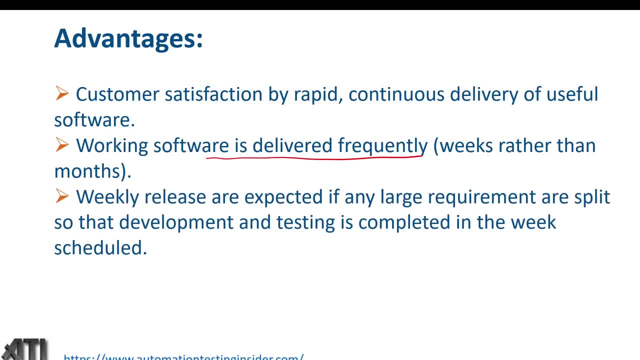 Quickly releases are expected if any large requirements are explained, so that development and testing is completed in the week scheduled. Customer developers and tester constantly interact with each other. These are some advantages of Agile development model. Daily cooperation between business people and developers: These are some advantages of Agile development model. 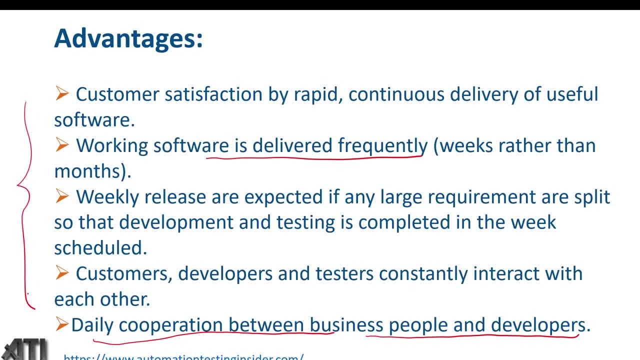 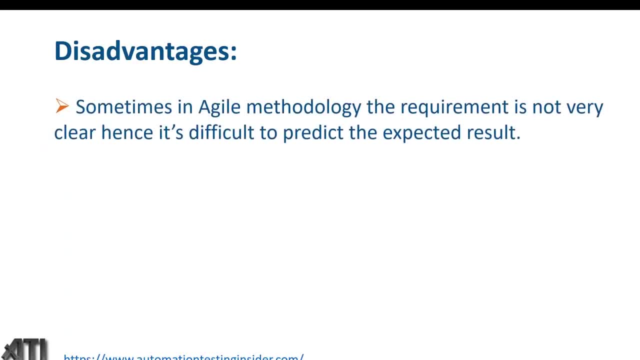 When we have such advantages, then we can deliver the software very frequently to the customer. Now let's talk about some of the disadvantages of Agile development model. Agile model: Sometimes in Agile methodology the requirements are not very clear, Hence it is difficult to predict the expected result.